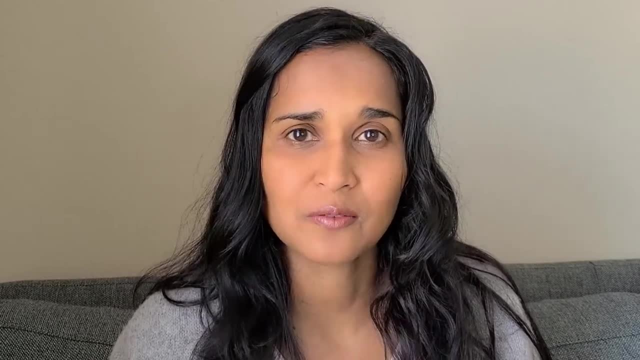 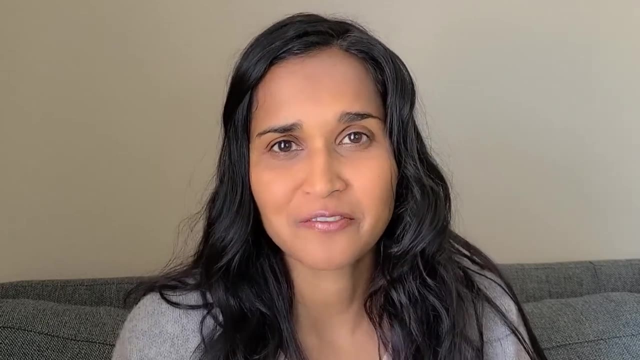 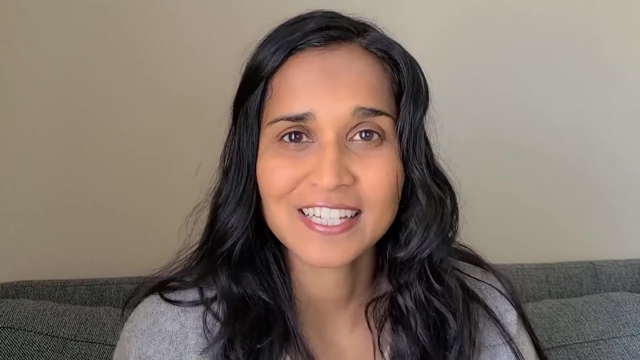 it's crucial to decide which types of mistakes you can better live with. To choose the right machine learning model and make informed decisions based on its predictions, it's important to understand the different measures of relevance. There are two measures of relevance that we're going to dive into in this video: precision and recall. So let's get into it. 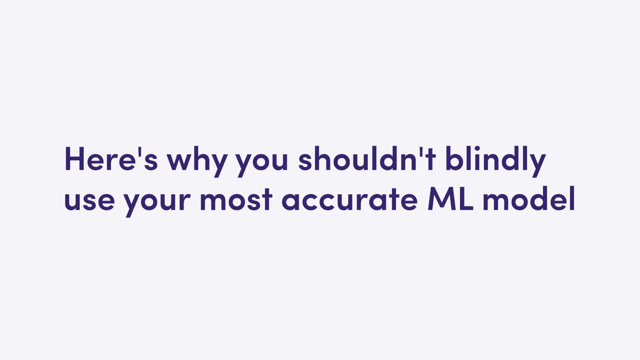 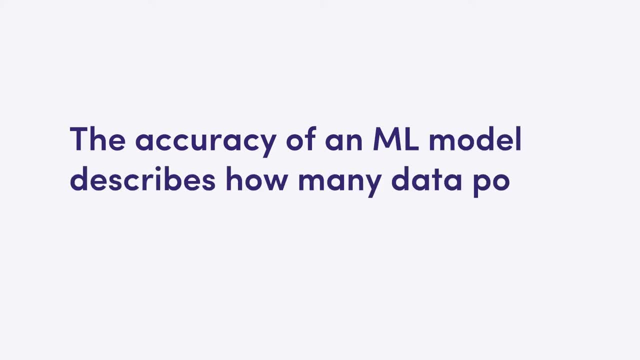 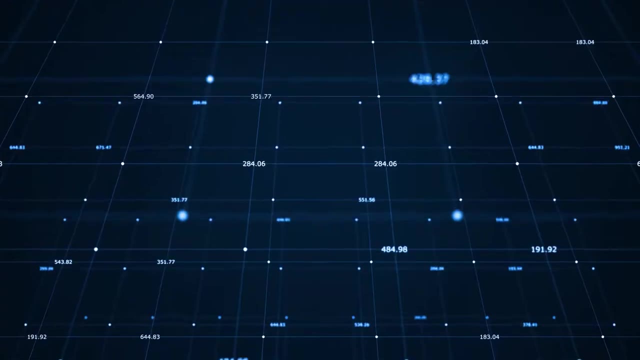 Here's why you shouldn't blindly use your most accurate machine learning model. First, let's start by defining accuracy. The accuracy of a machine learning model describes how many data points were detected correctly. To use a practical example, let's look at an image classification problem in which the AI is tasked to label. 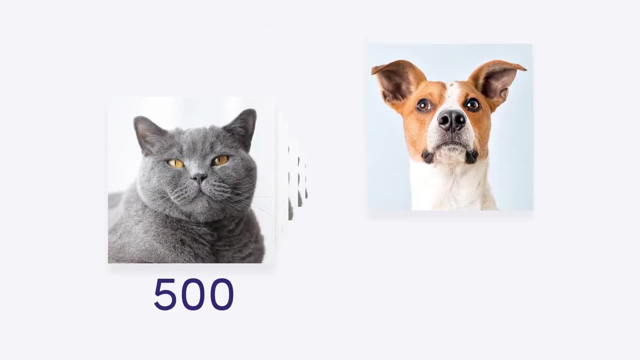 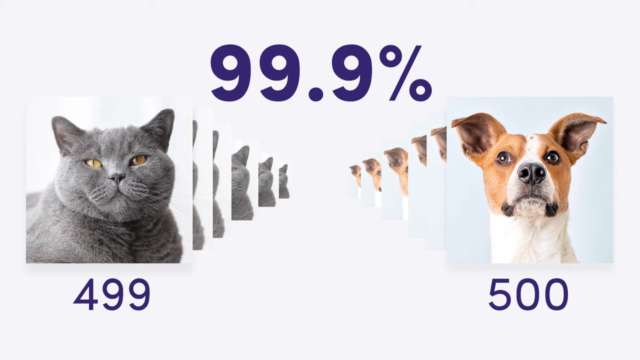 an image dataset containing images of 500 cats and 500 dogs. The model correctly labels 500 dogs and 499 cats. Mistakenly it labels one cat as dog. The corresponding accuracy is therefore 99.9% Here. accuracy is a good assessment of model quality. For comparison, let's look at a second. 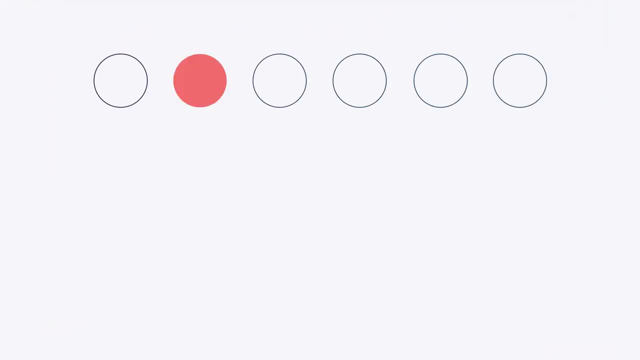 less balanced example. A hospital looks for cancer in 1,000 images. In reality, two of those pictures contain evidence for cancer. but the other two images contain evidence for cancer, The model only detects one of them. Since the model only makes one mistake by labeling one, 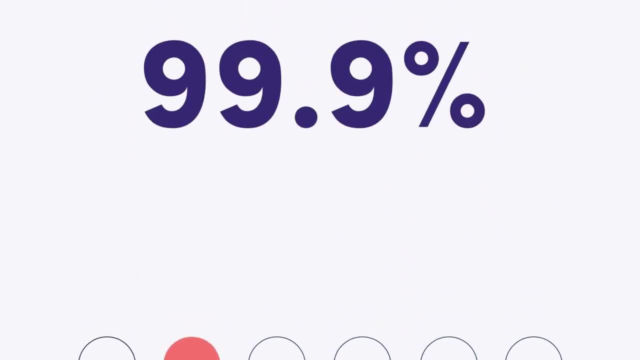 cancerous image as healthy. the accuracy of the model is also at 99.9%. In this case, the 99.9% accuracy gives us a wrong impression, as the model actually missed 50% of relevant items. Out of doubt, it would be preferable to reduce the accuracy to 99% and mistakenly detect eight. 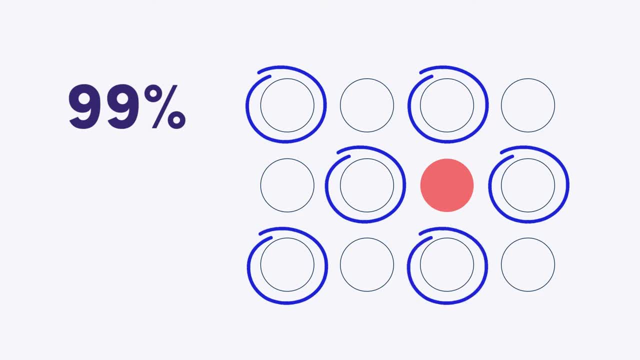 healthy images as cancerous. If, in return, the second cancerous image is healthy, the model could be detected. The trade-off of manually checking 10 images to discover two relevant elements is unworthy of discussion, But how can you formalize this when choosing your ML model? 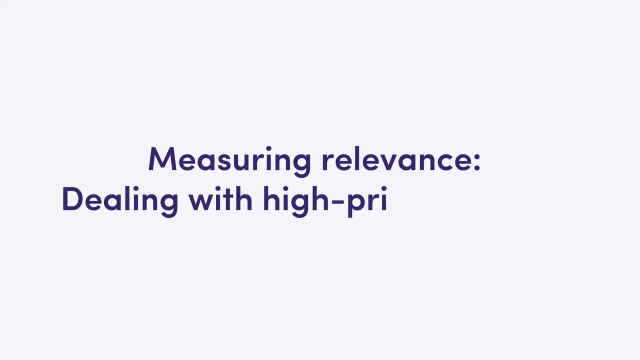 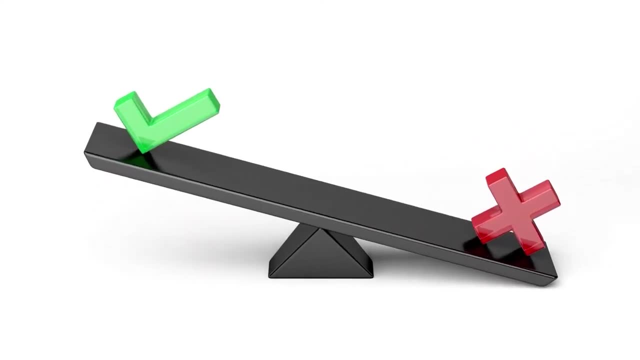 Let's dive deeper: Measure in relevance, dealing with high-priority classes. If your dataset is not well balanced or mistakes have varying impact, your model's accuracy is not a good measure for performance. Whenever you are looking for specific information, the main task is often to differentiate. 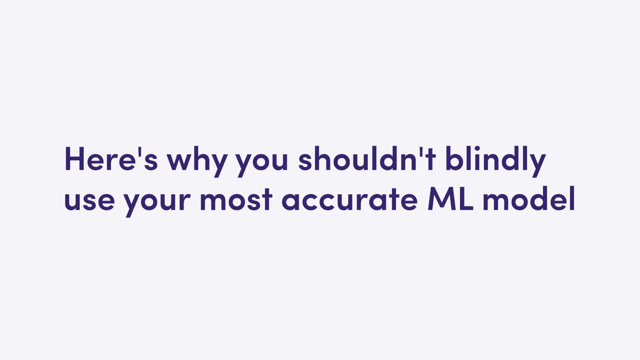 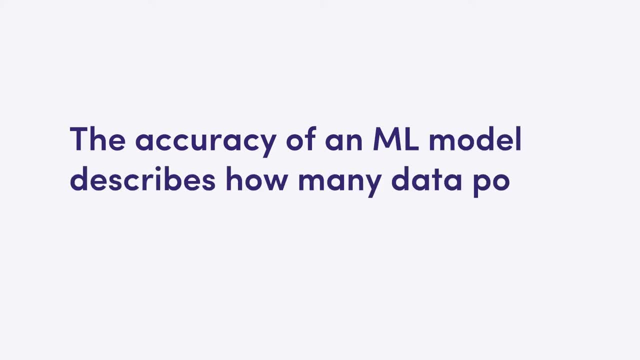 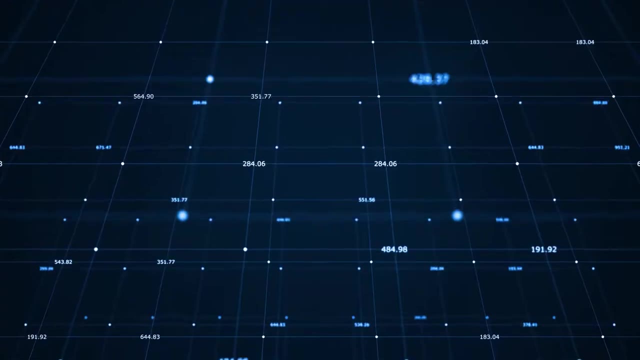 Here's why you shouldn't blindly use your most accurate machine learning model. First, let's start by defining accuracy. The accuracy of a machine learning model describes how many data points were detected correctly. To use a practical example, let's look at an image classification problem in which the AI is tasked to label. 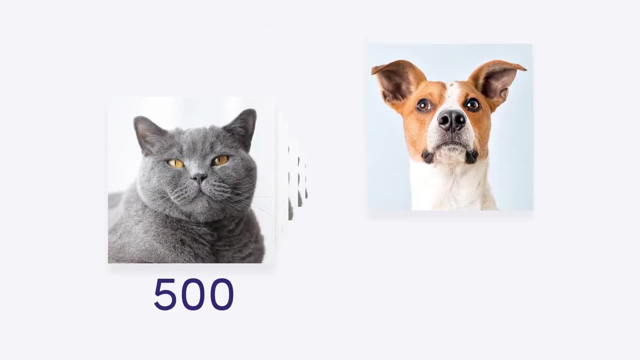 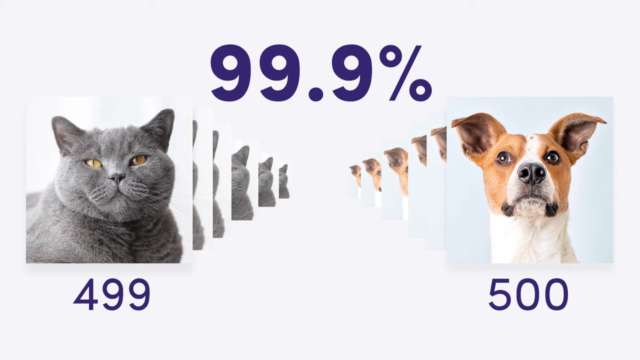 an image dataset containing images of 500 cats and 500 dogs. The model correctly labels 500 dogs and 499 cats. Mistakenly it labels one cat as dog. The corresponding accuracy is therefore 99.9% Here. accuracy is a good assessment of model quality. For comparison, let's look at a second. 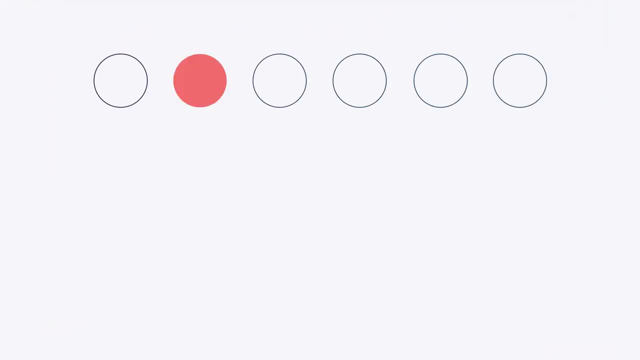 less balanced example. A hospital looks for cancer in 1,000 images. In reality, two of those pictures contain evidence for cancer. but the other two images contain evidence for cancer, The model only detects one of them. Since the model only makes one mistake by labeling one, 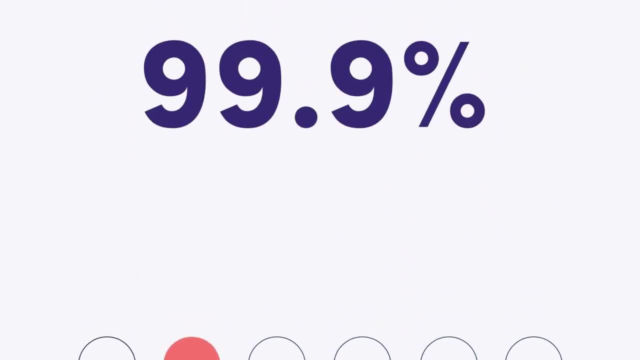 cancerous image as healthy. the accuracy of the model is also at 99.9%. In this case, the 99.9% accuracy gives us a wrong impression, as the model actually missed 50% of relevant items. Out of doubt, it would be preferable to reduce the accuracy to 99% and mistakenly detect eight. 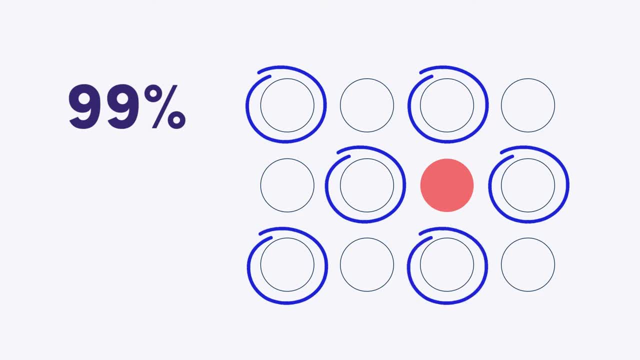 healthy images as cancerous. If, in return, the second cancerous image is healthy, the model could be detected. The trade-off of manually checking 10 images to discover two relevant elements is unworthy of discussion, But how can you formalize this when choosing your ML model? 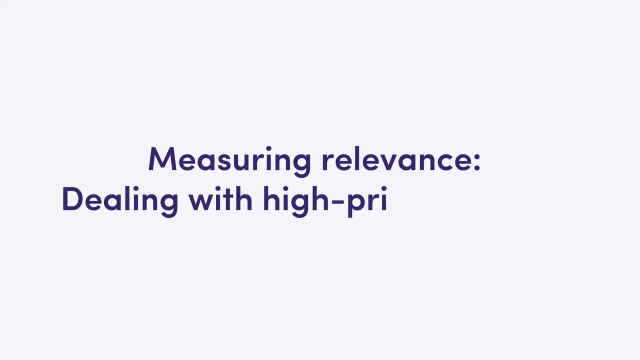 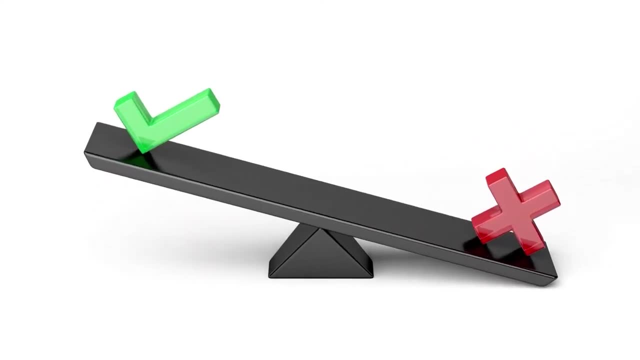 Let's dive deeper: Measure in relevance, dealing with high-priority classes. If your dataset is not well balanced or mistakes have varying impact, your model's accuracy is not a good measure for performance. Whenever you are looking for specific information, the main task is often to differentiate. 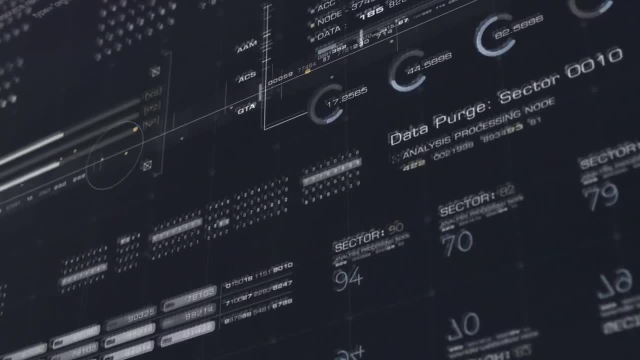 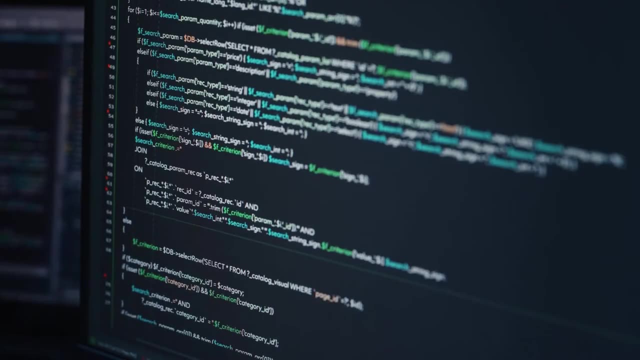 between the relevant data and the unbalanced data. If you are looking for specific information, you are looking for the data you are looking for and the irrelevant information that clouds your view. Therefore, it is more important to analyze model performance concerning relevant elements and not the overall dataset. Let's look at our first example. If the objective is to detect dogs, 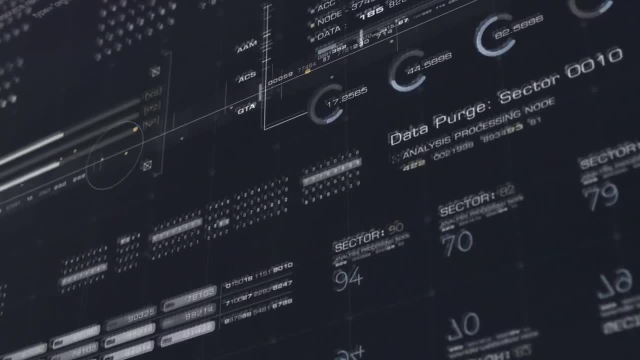 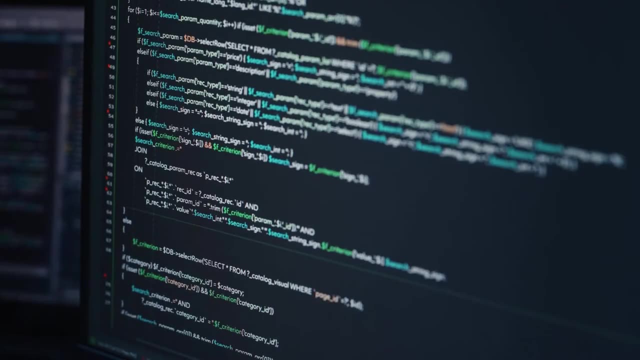 between the relevant data and the unbalanced data. If you are looking for specific information, you are looking for the data you are looking for and the irrelevant information that clouds your view. Therefore, it is more important to analyze model performance concerning relevant elements and not the overall dataset. Let's look at our first example. If the objective is to detect dogs, 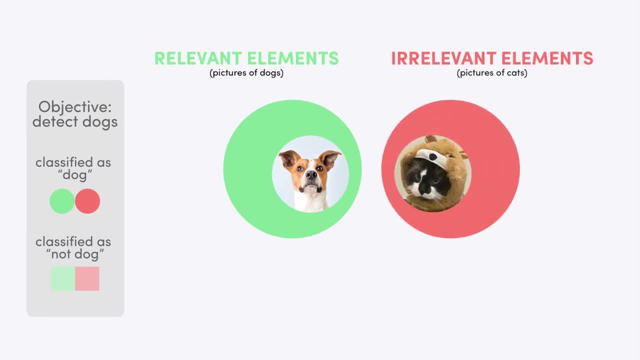 all dogs are relevant elements, whereas cats are irrelevant elements. In this task, the AI can make two types of mistakes: It can miss a detection of a dog, false, negative, or it can wrongly identify a cat as a dog. If the objective is to detect dogs, all dogs are irrelevant elements, whereas cats are. 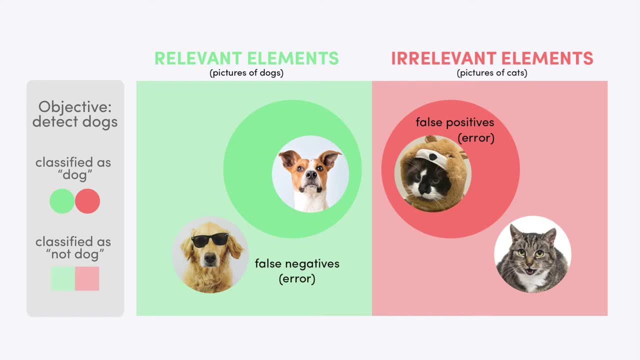 relevant elements. It can miss a detection of a dog: false positive. This matrix of choices shows the true positives, false negatives, false positives and true negatives that are possible. Ideally, the AI should detect all dogs without a miss and make no mistake by labeling a cat as a. 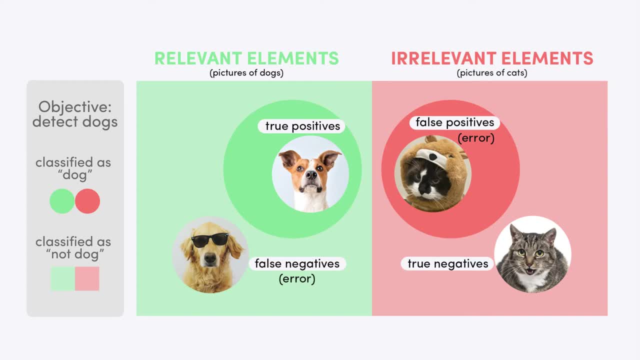 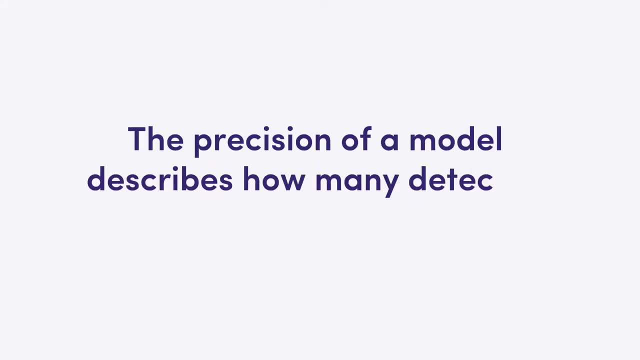 dog. Hence, there are two main dimensions according to which the correctness of machine learning models can be compared: Precision: The precision of a model describes how many detected items are relevant. If the objective is to detect dogs, all dogs are relevant elements, whereas cats are. 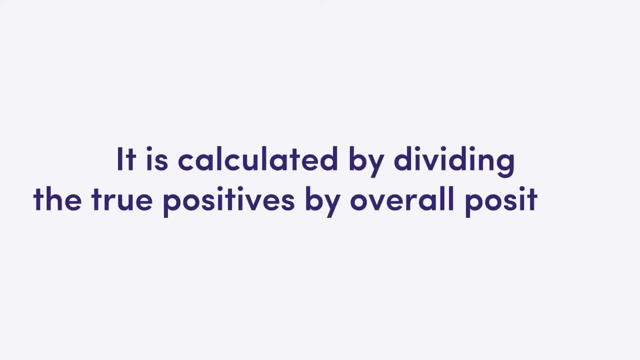 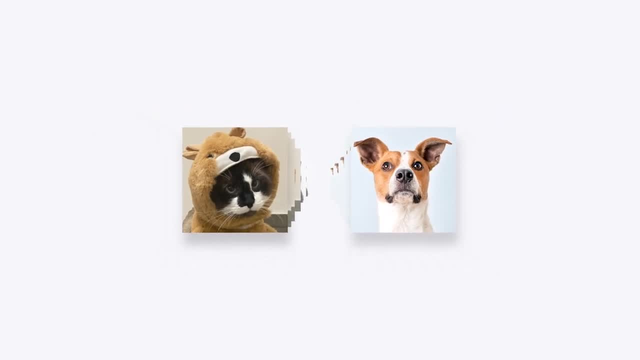 relevant elements. It is calculated by dividing the true positives by overall positives. In our first example, it compares the number of dogs that were detected to the number of dogs and dressed-up cats that were all detected as dogs. Since missed detections of dogs are not considered in the 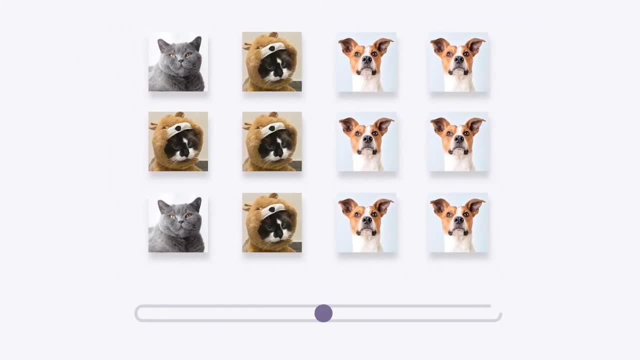 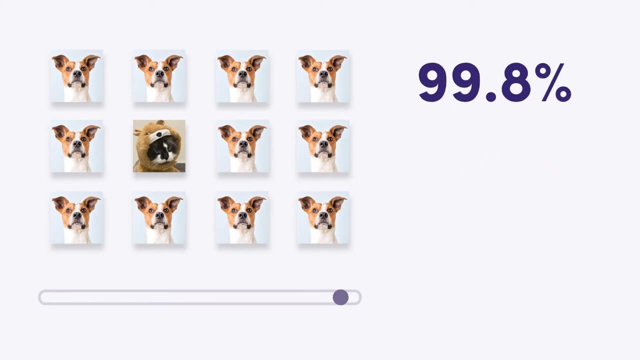 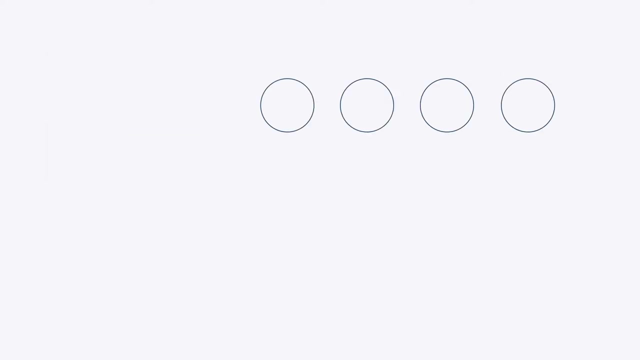 calculation. it can be increased by setting higher thresholds on when a dog should be detected as such. In the cat-dog example, the precision is at 99.8%, since out of the 501 animals that were detected as dogs, only one was a cat. If we look at the cancer example, we get a perfect score of 100%. 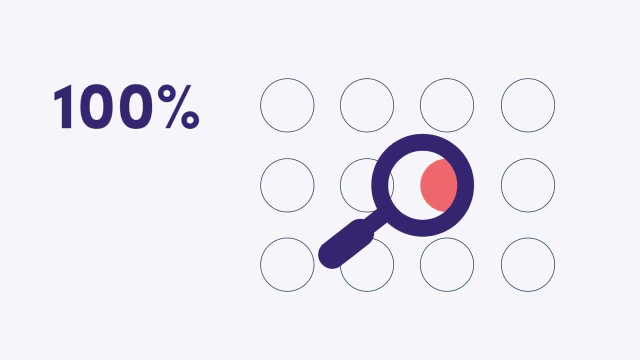 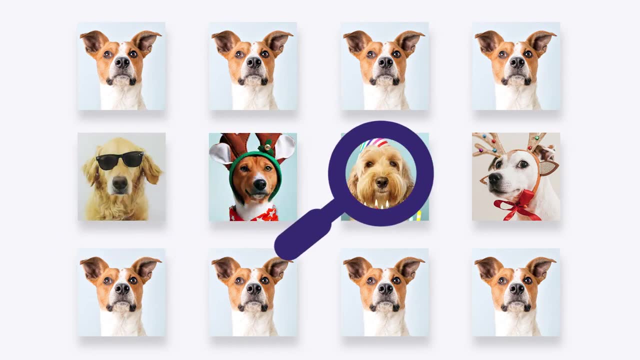 since the model detected no healthy image as cancerous. Besides being a measure of model performance, precision can be seen as the probability that a randomly selected item which is labeled as relevant is a true positive. In the cancer example, the precision percentage can be: 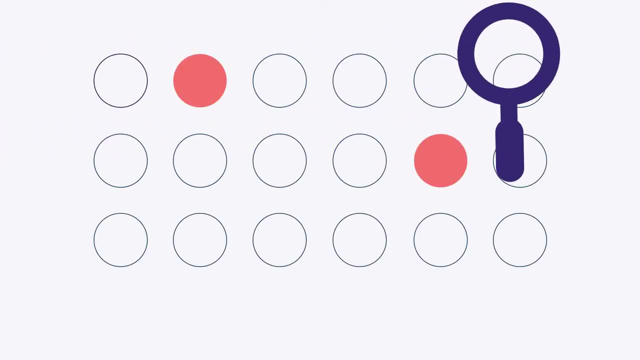 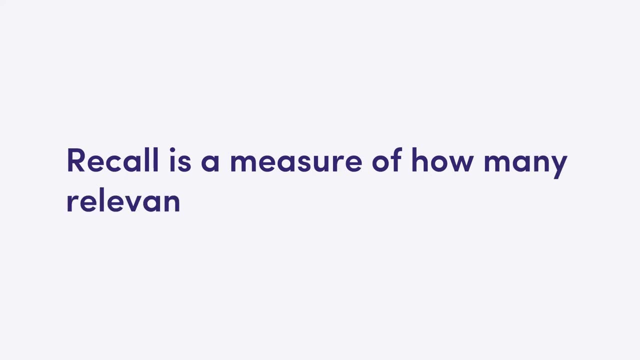 translated as the probability that an image which the model detected as cancerous actually shows cancer Recall. Recall is the measure of how many relevant elements were detected. Therefore, it divides the true positives by the number of relevant elements. In our cat-dog example, it compares the dogs that were detected to the overall amount of. 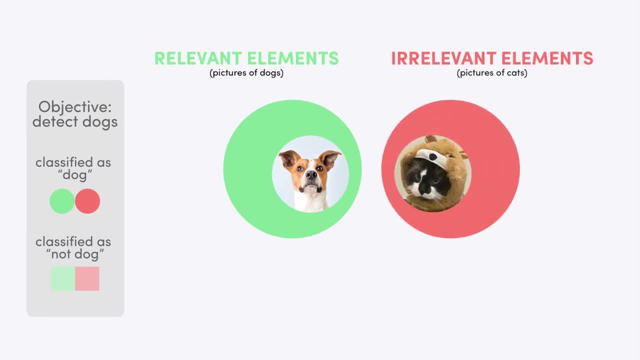 all dogs are relevant elements, whereas cats are irrelevant elements. In this task, the AI can make two types of mistakes: It can miss a detection of a dog, false, negative, or it can wrongly identify a cat as a dog. If the objective is to detect dogs, all dogs are irrelevant elements, whereas cats are. 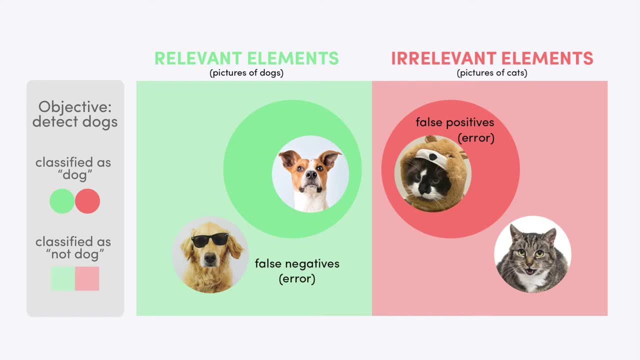 relevant elements. It can miss a detection of a dog: false positive. This matrix of choices shows the true positives, false negatives, false positives and true negatives that are possible. Ideally, the AI should detect all dogs without a miss and make no mistake by labeling a cat as a. 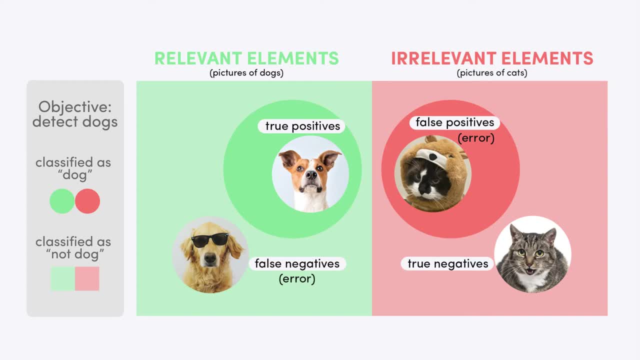 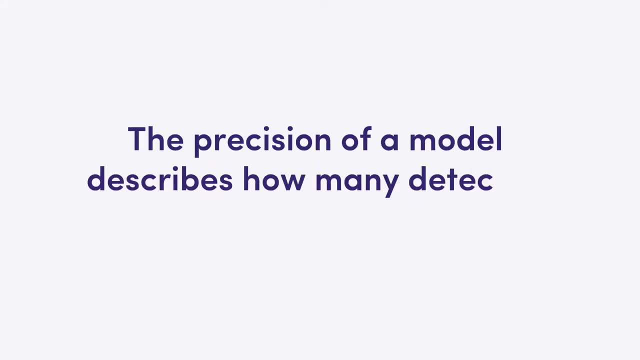 dog. Hence, there are two main dimensions according to which the correctness of machine learning models can be compared: Precision: The precision of a model describes how many detected items are relevant. If the objective is to detect dogs, all dogs are relevant elements, whereas cats are. 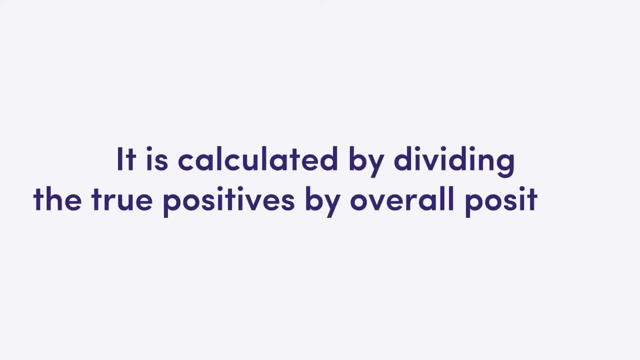 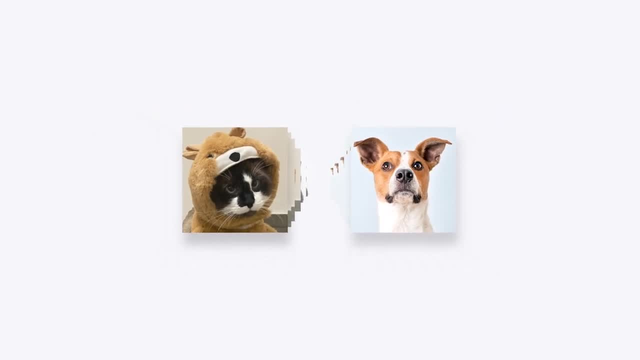 relevant elements. It is calculated by dividing the true positives by overall positives. In our first example, it compares the number of dogs that were detected to the number of dogs and dressed-up cats that were all detected as dogs. Since missed detections of dogs are not considered in the 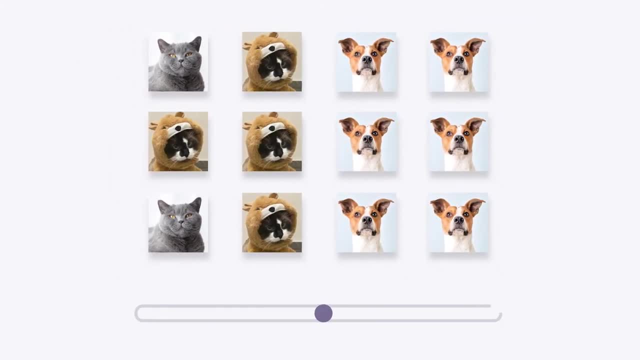 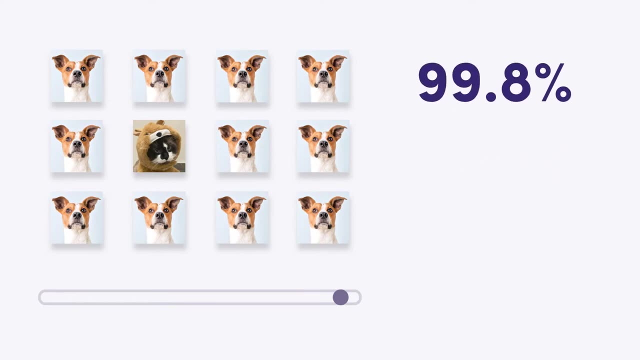 calculation. it can be increased by setting higher thresholds on when a dog should be detected as such. In the cat-dog example, the precision is at 99.8%, since, out of the 501 animals that were detected as dogs, the precision is at 99.8%. If the objective is to detect dogs, all dogs are relevant. 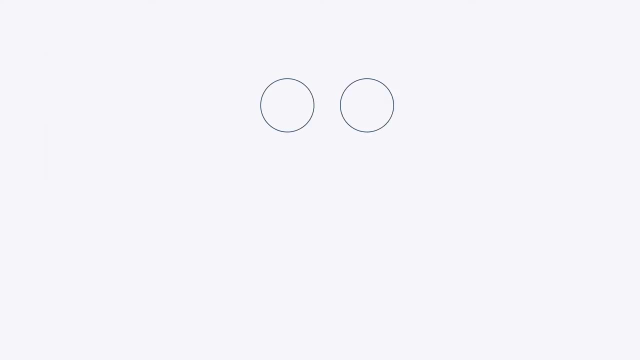 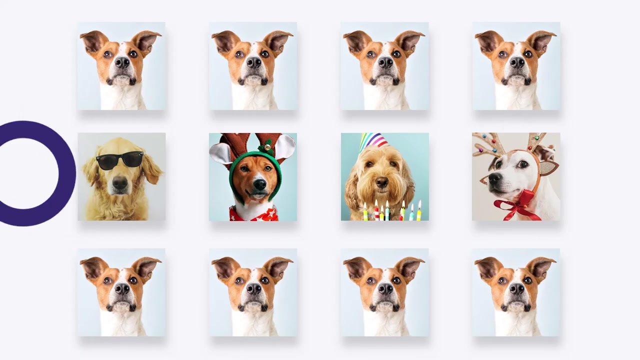 elements, Since missed detections of dogs are not considered as dogs. only one was a cat. If we look at the cancer example, we get a perfect score of 100%, since the model detected no healthy image as cancerous. Besides being a measure of model performance, precision can be seen as the 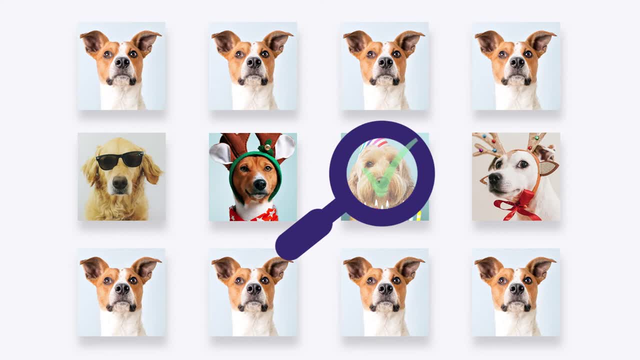 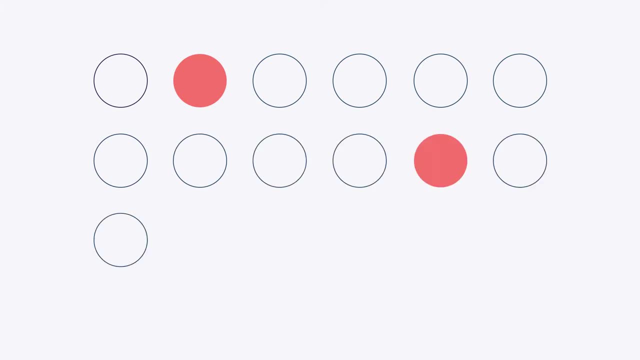 probability that a randomly selected item which is labeled as relevant is a true positive. In the cancer example, the precision percentage can be translated as the probability that an image which the model detected as cancerous actually shows cancer Recall. Recall is the measure of how many relevant. 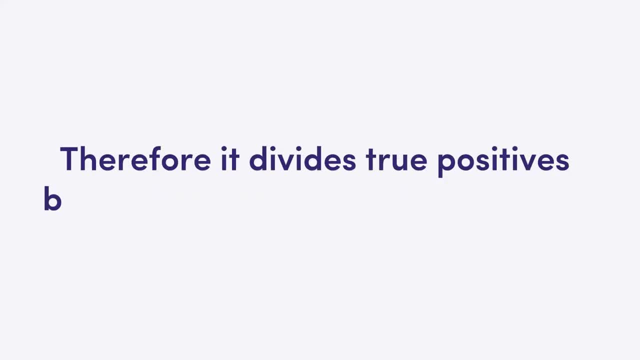 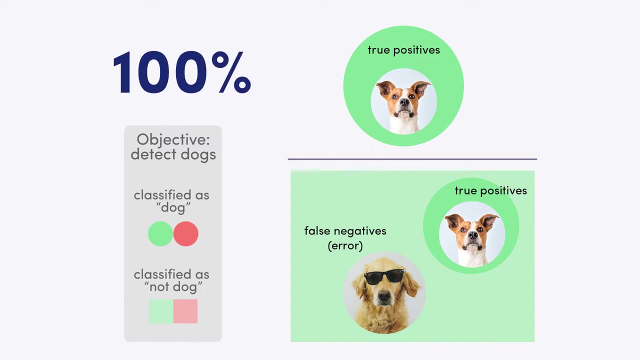 elements were detected. Therefore it divides true positives by the number of relevant elements. In our cat-dog example, it compares the dogs that were detected to the overall amount of dogs in the dataset, disguised or not. Hence the recall of the model is at a perfect 100%. In contrast, 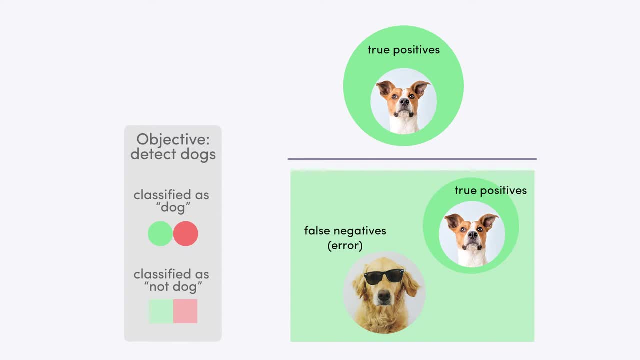 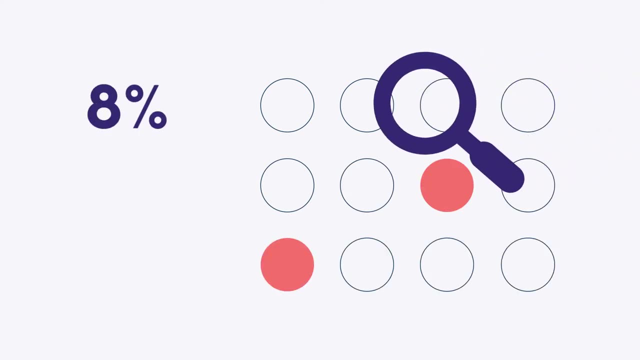 dogs in the data set, disguised or not. Hence the recall of the model is at a perfect 100%. In contrast, the cancer detection model has a terrible recall, Since only one of two examples of cancer were detected. the total number of he-eaters atいて hospital. 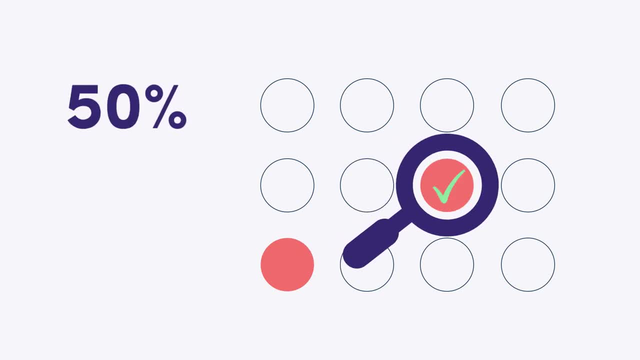 is at an incredible four percent, Since only one of two examples of cancer were detected. then there is an toasted risk forgetting. return to the backgroundul. the recall is at 50%, While accuracy and precision suggested that the model is suitable to detect cancer, calculating recall reveals its weakness, As with precision, analysing purely recall can. 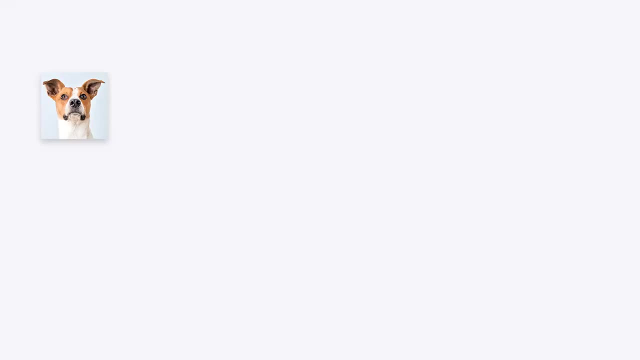 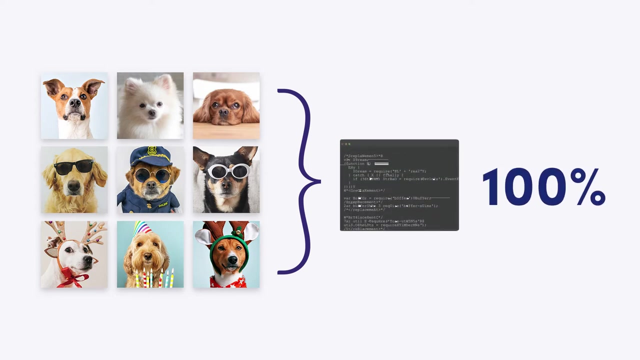 also give us a wrong impression of model performance. A model labelling all animals in the dataset as dog would have a recall of 100%, since it would detect all dogs without a miss. The 500 wrongly labelled cats would not have an impact on recall For the individual element. 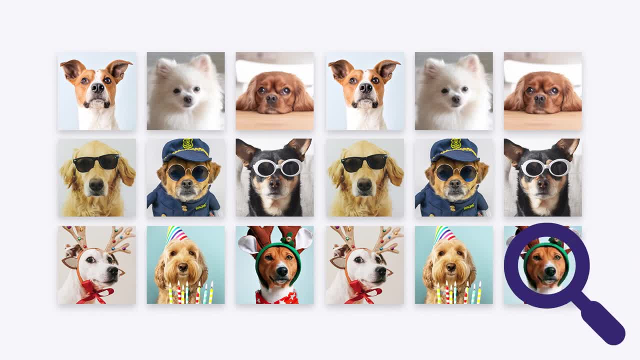 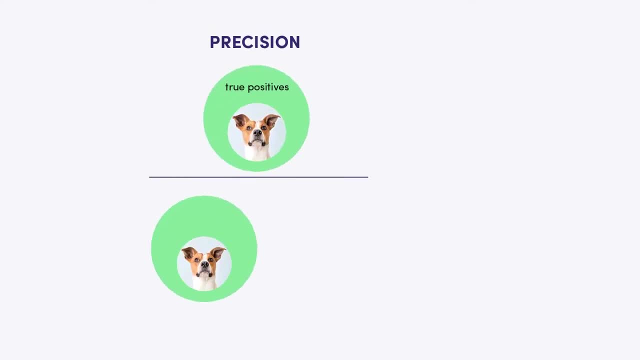 the recall percentage gives the probability that a randomly selected relevant item from the dataset will be detected. This is how precision and recall are calculated. Going back to the question of how to select the right model, there's a trade-off between trying to detect all relevant items. 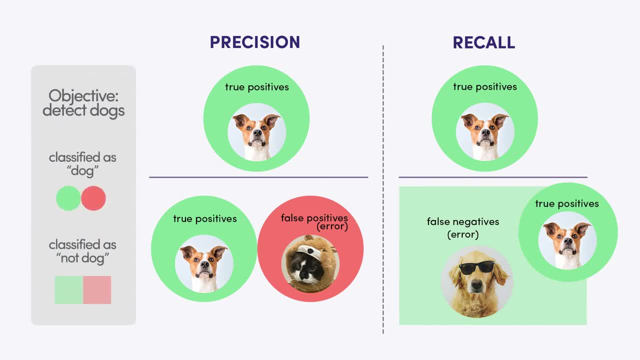 and avoiding making wrong detections. In the end, the decision depends on your use case. Put differently, you will need to consider these questions: How crucial is it that you detect every relevant element? Are you willing to manually sort out irrelevant elements in return for optimal recall? 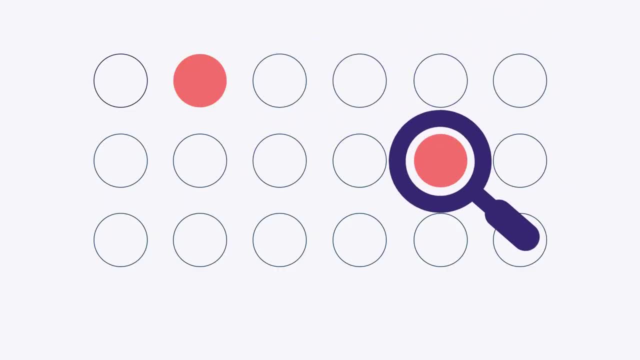 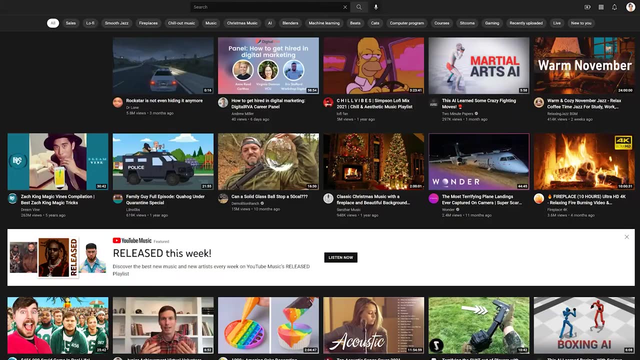 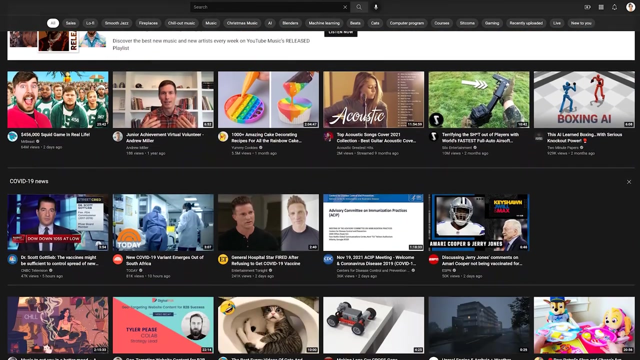 In the cancer diagnosis examples. false negatives should be avoided at all costs, since they have lethal consequences. Here. recall is a better measure than precision If you were to optimise recommendations on YouTubes. false negatives are less important, since only a small subset of recommendations is shown anyways. 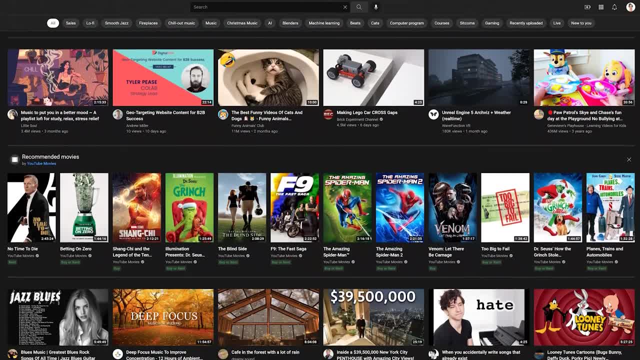 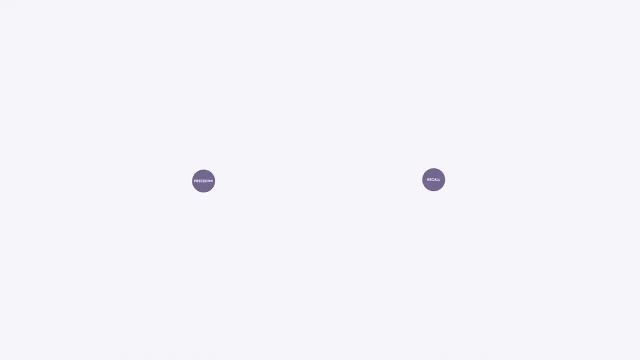 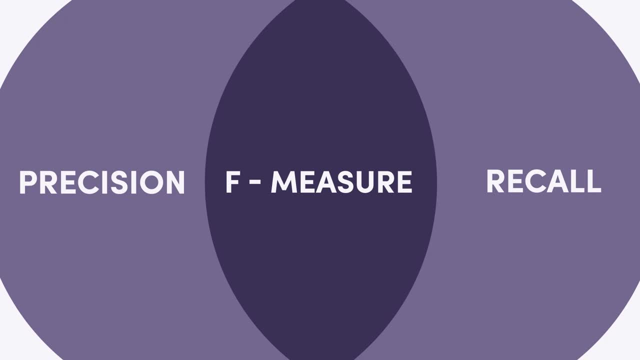 More importantly, false positives, bad recommendations, should be avoided. Hence the model should be optimised for precision. What is the F-measure? in machine learning, There is also a way to combine both precision and recall, and it can sometimes make sense to calculate what's called the F-measure. 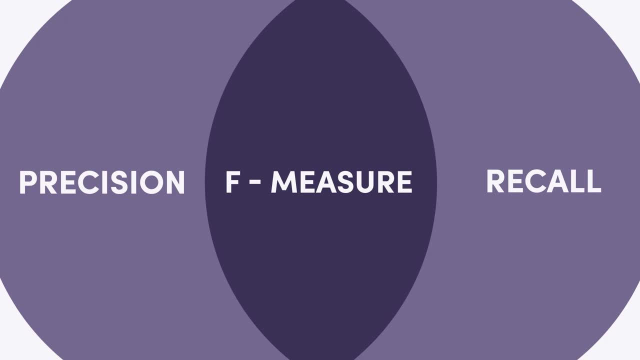 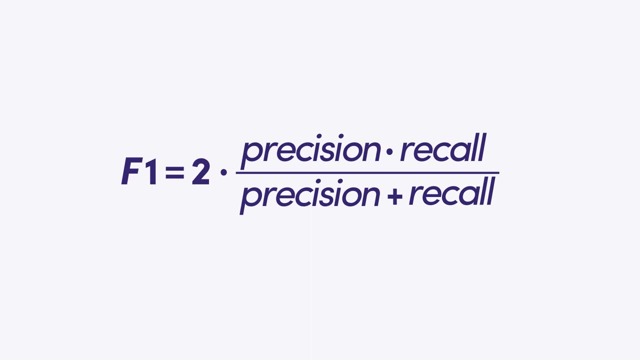 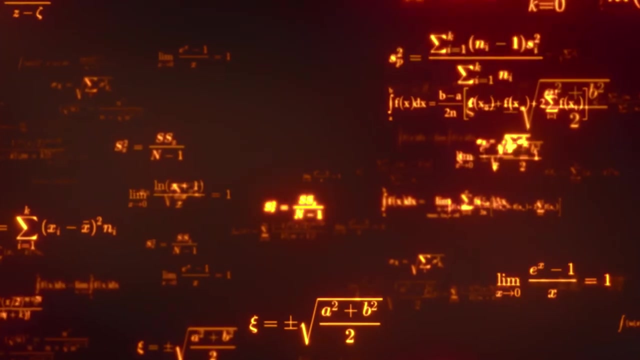 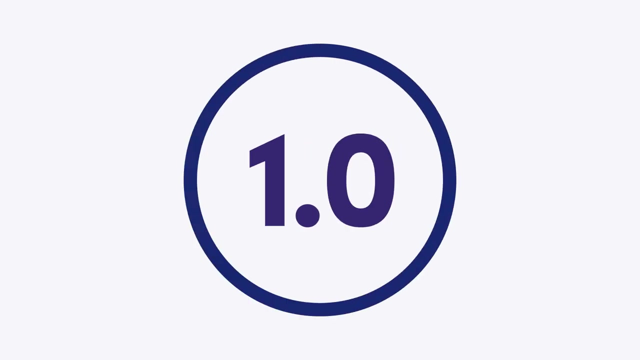 This provides both techniques into a single measure with each side. given the proper weighting, The equation looks like this: The equation for determining the F-measure is the harmonic mean of the two fractions for precision and recall. The result is a value between 0.0 for the worst and 1.0 for the best F-measure. 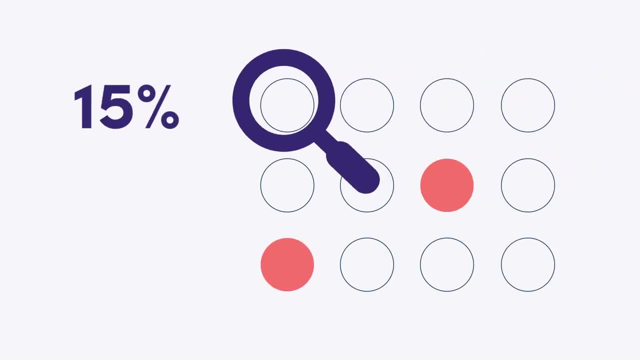 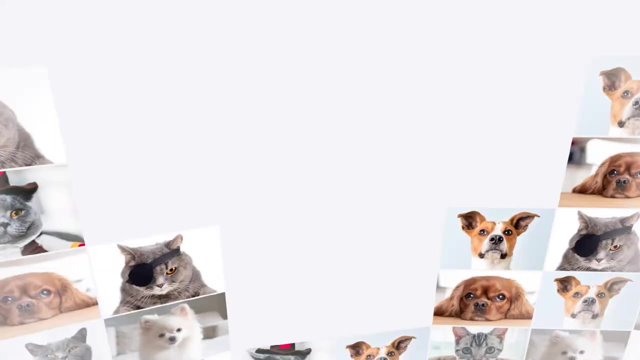 the cancer detection model has a terrible recall, Since only one of two examples of cancer were detected. the recall is at 50%. While accuracy and precision suggested that the model is suitable to detect cancer, calculating recall reveals its weakness, As with precision, analyzing purely. 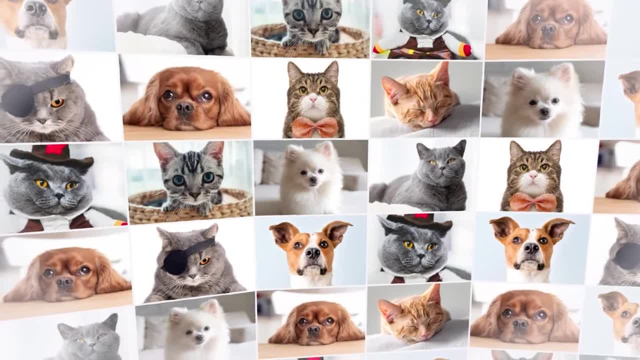 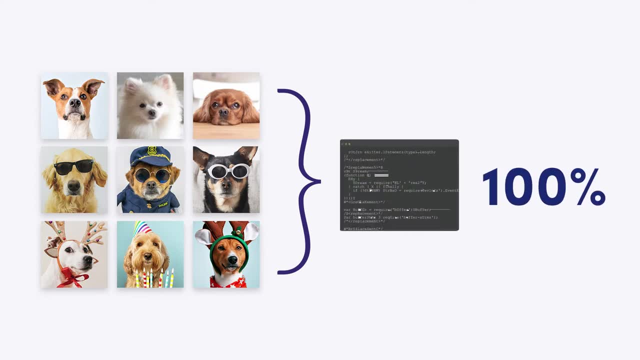 recall can also give us a wrong impression of model performance. A model labeling all animals in the dataset as dog would have a recall of 100%, since it would detect all dogs without a miss. The 500 wrongly labeled cats would not have an impact on recall. When documenting deaths. workunosphite often affect animals such as cats, dogs and cats. Brอะdnāt patients usually arePE我们 them走在 驼per case because dog null cane disease or any grcase from Nurse Cat Santa第二個. the cats don't have a response too. 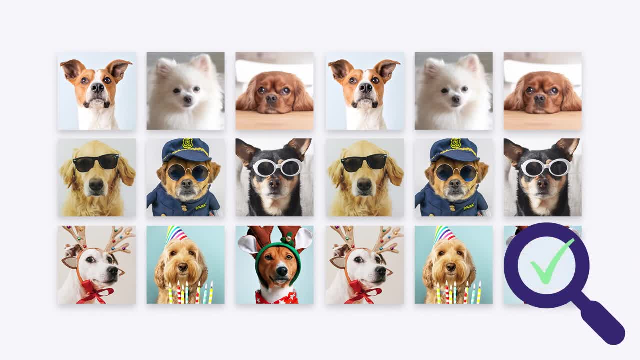 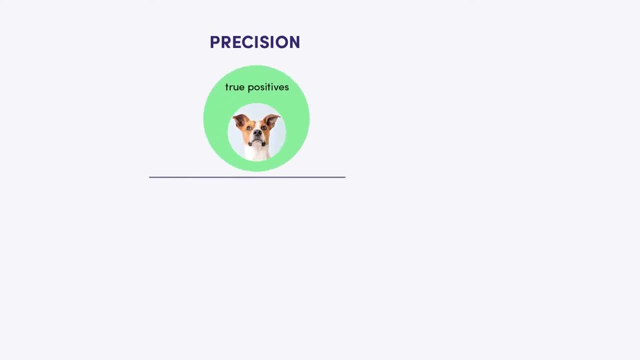 element, the recall percentage, gives the probability that a randomly selected relevant item from the data set will be detected. This is how precision and recall are calculated. Going back to the question of how to select the right model, there's a trade-off between trying to detect all relevant items and 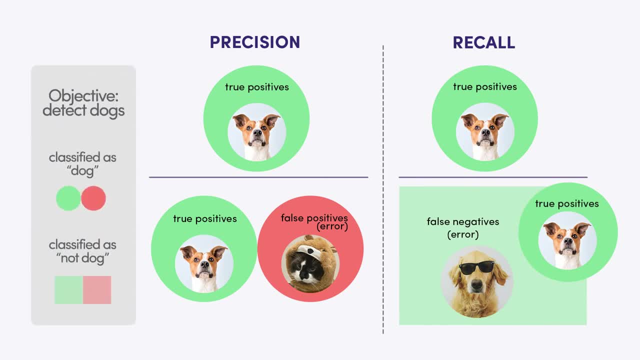 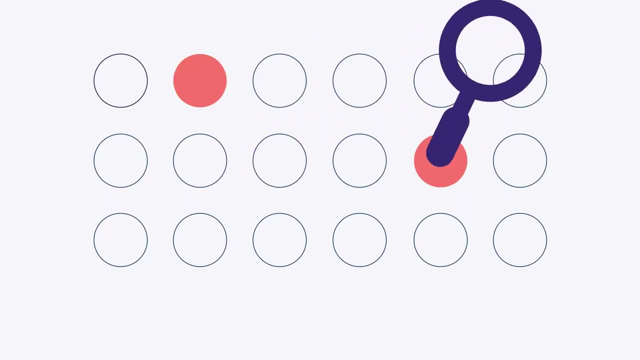 avoiding making wrong detections. In the end, the decision depends on your use case. Put differently, you will need to consider these questions: How crucial is it that you detect every relevant element? Are you willing to manually sort out irrelevant elements in return for optimal recall In the cancer? 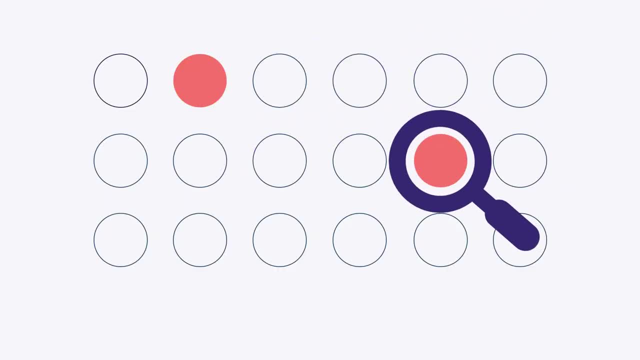 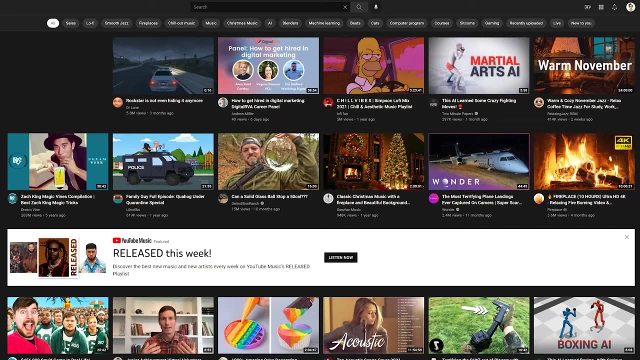 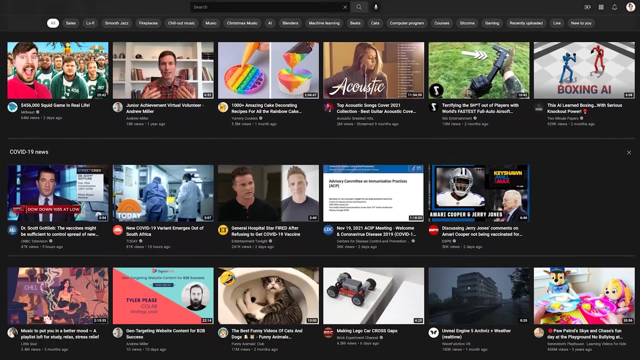 diagnosis examples. false negatives should be avoided at all costs, since they have lethal consequences. Here, recall is a better measure than precision If you were to optimize recommendations on YouTube's. false negatives are less important, since only a small subset of recommendations is shown anyways. More importantly, false positives- bad recommendations. 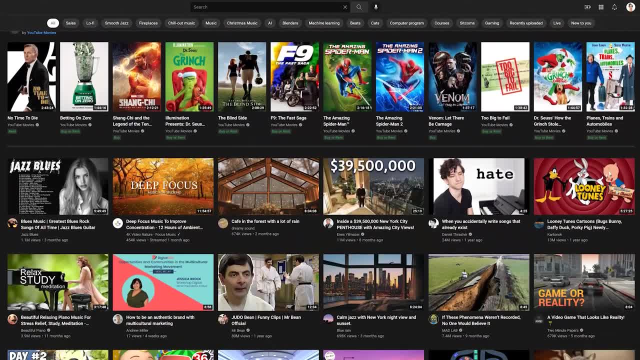 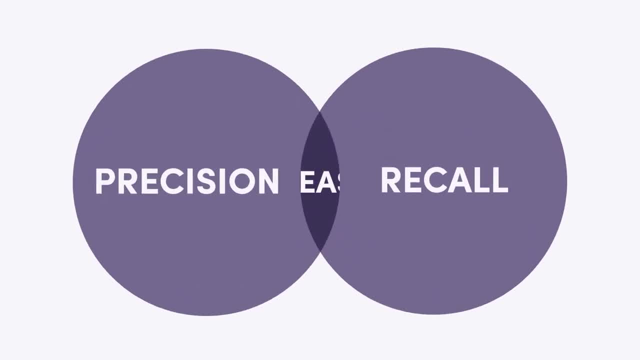 and false negatives are less important. More importantly, false positives, bad recommendations, should be avoided. Hence the model should be optimized for precision. What is the F-measure? in machine learning, There is also a way to combine both precision and recall, and it can sometimes make sense to calculate. 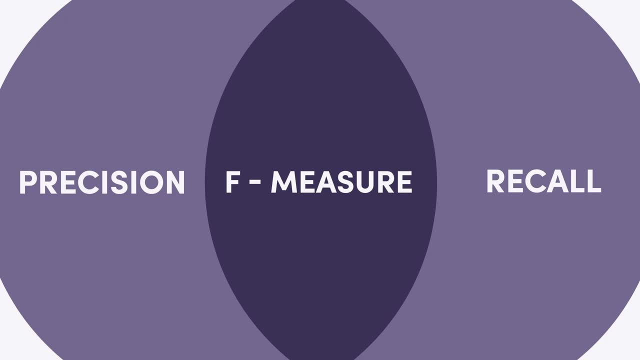 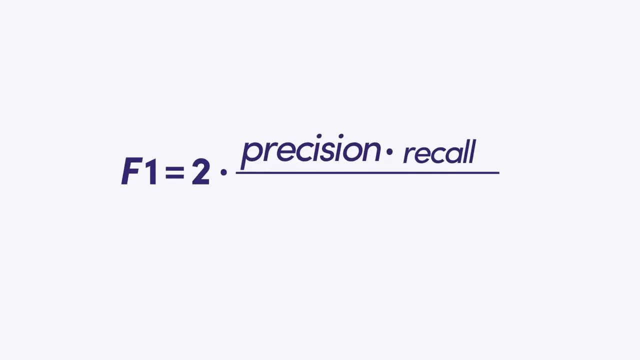 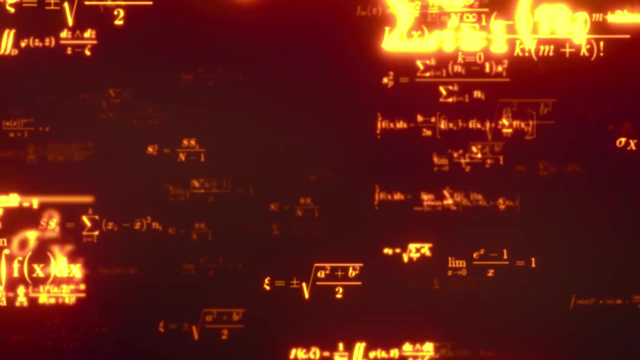 what's called the F-measure. This provides both techniques into a single measure. with each side given the proper weighting. The equation looks like this: The equation for determining the F-measure in machine learning is the following: The F-measure is the harmonic mean of the two fractions for precision and recall. 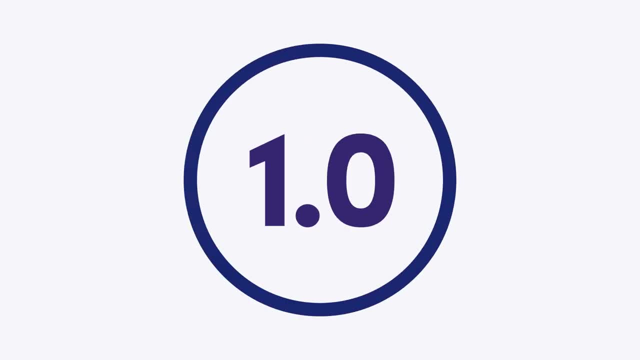 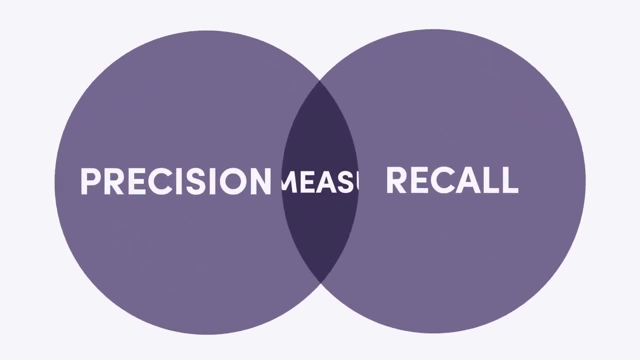 The result is a value between 0.0 for the worst and 1.0 for the best F-measure. Another way of weighting the algorithms is using the F-beta measure, which acts as a generalization of the F-measure, with the addition of a configuration. 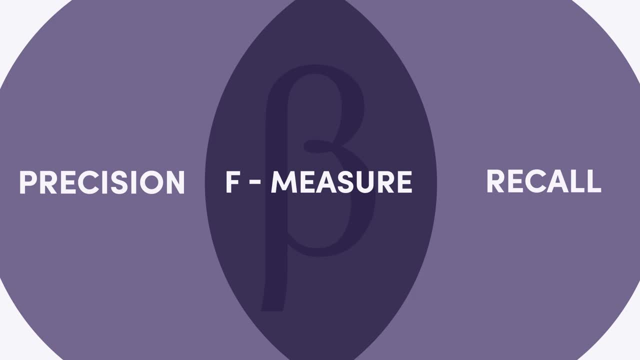 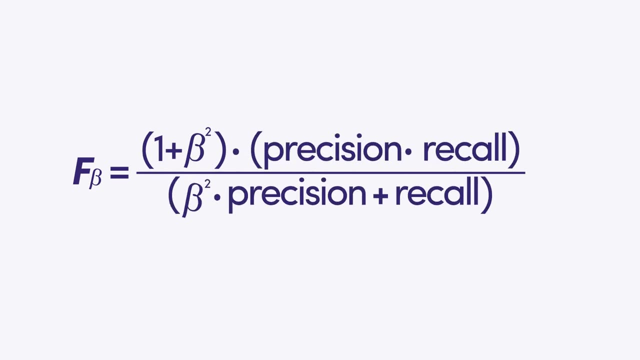 parameter, the beta, in which the harmonic mean is controlled by a coefficient. The F-beta measure looks like this To summarize. To summarize the main points: precision quantifies the number of positive class predictions that actually belong to the positive class Recall. 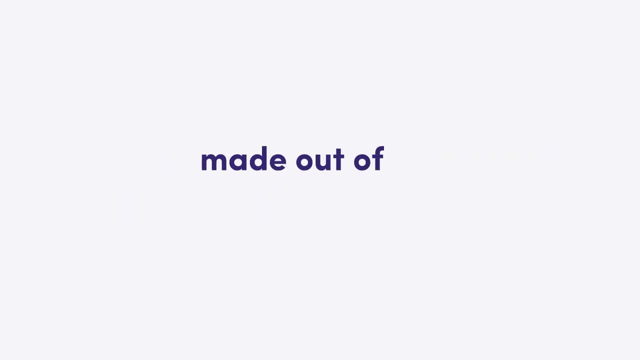 quantifies the number of positive class predictions made out of all positive examples in the data set. The F-measure provides a single score that balances both the concerns of the precision and recall in one number. Thank you for watching and see you in the next one. Subtitles by the Amaraorg community.